the weak nuclear force and the Higgs boson, which is responsible for giving mass to all the mass matter. In addition, bosons have a spin that is classified with an integer, and multiple boson particles can be in the same place, at the same time, in the same quantum state. 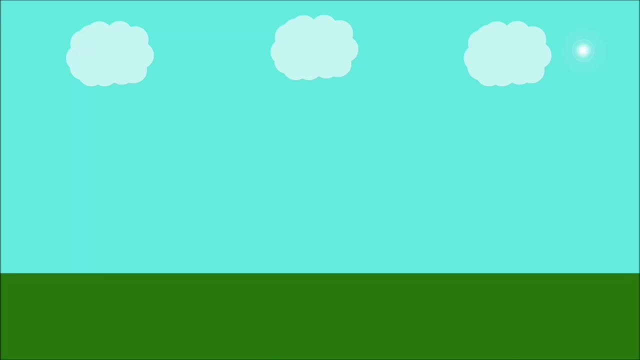 So, now that you kinda know what the standard model is, you're probably wondering what could be wrong with the standard model. After all, it seems like a pretty good explanation of our universe, right? Well, for starters, physicists claim that the standard model is. 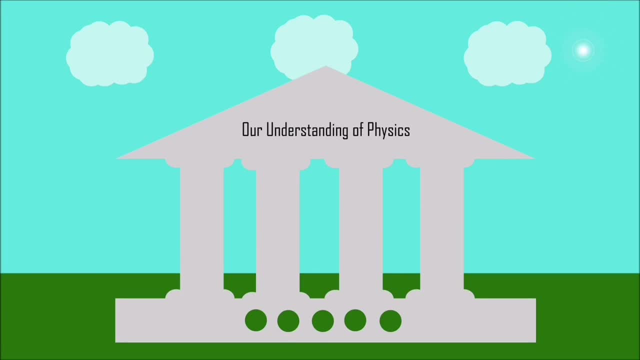 unfinished. so physicists proposed the idea of supersymmetry, saying that for every particle in the standard model there was a heavier partner particle with a spin varying about one half, with the goal of filling in some of the holes of the standard model. But there 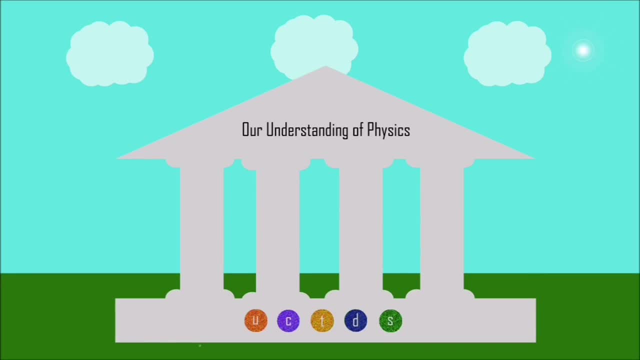 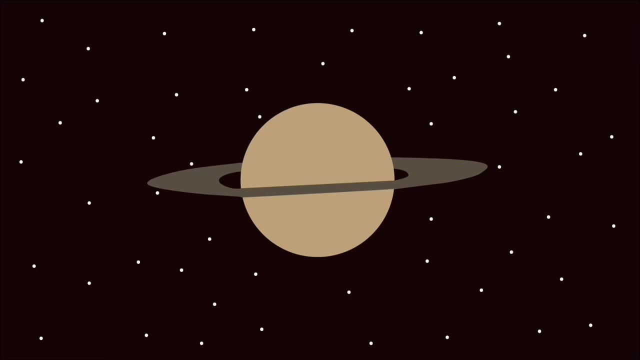 are some other problems which supersymmetry can help us solve, but unfortunately, due to time constraints, we can only look at two of the most arguably important issues in physics which supersymmetry helps us solve. The first problem supersymmetry helps solve is the issue of the Higgs boson. But first, 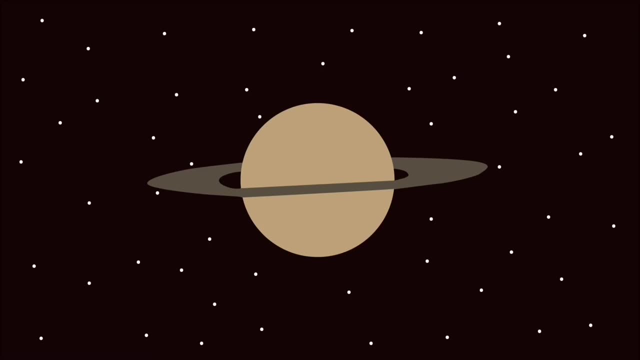 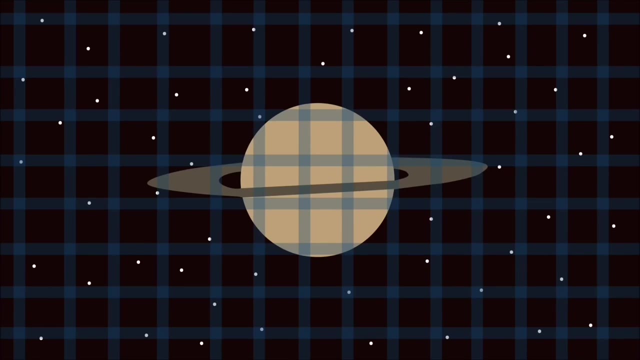 of all, what is the Higgs boson? Well, throughout the universe, an entity called the Higgs field permeates. When particles move through this field, they interact with it, and this interaction with this field is what gives particles and matter its mass. The Higgs field consists. 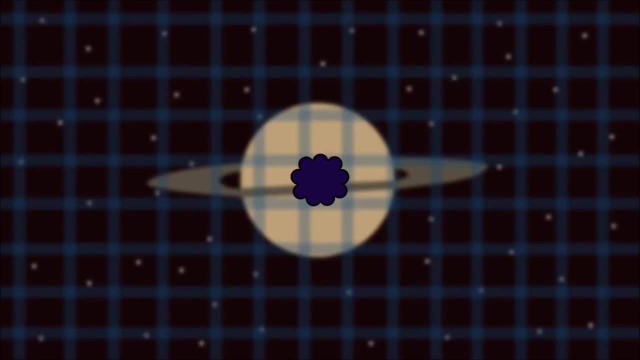 of a subatomic particle known as the Higgs boson. Physicists say the Higgs boson is not very heavy. However, this seems surprising, as physicists also state that the interaction between the Higgs and the subatomic particles in the standard model would mean a heavy Higgs boson. However, to quote an article from CERN which explains it perfectly, the extra particles predicted by supersymmetry would cancel out the contributions to the Higgs mass from their standard model partners, making a light Higgs boson possible. 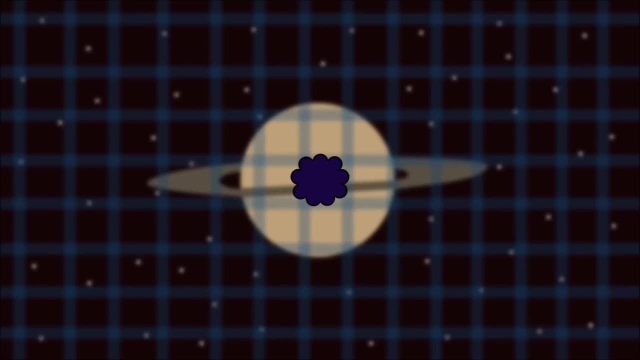 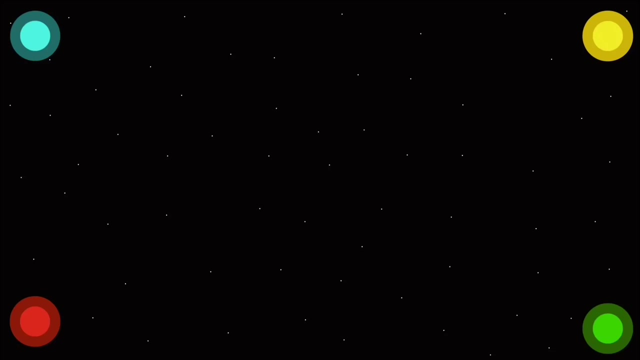 Now let's take a look at the second problem. supersymmetry solves the issue of grand unification theory. Today, it seems that the fundamental forces seem separate. However, just a fraction of a second after the big bang, the four forces that we know today were unified into a single. 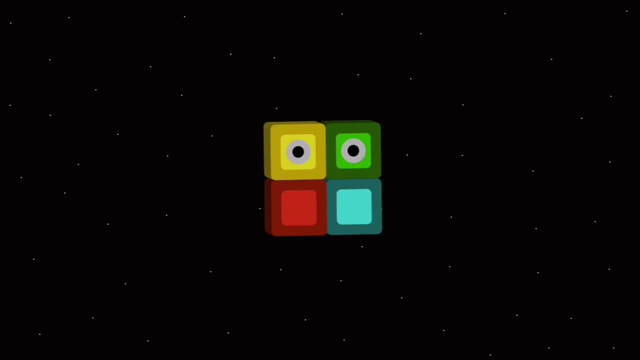 force. However, as the universe cooled down the forces separated into the four distinct forces we know and love today. Well, the same article from CERN also claims, and I quote: if supersymmetric particles were included in the standard model, the interactions of 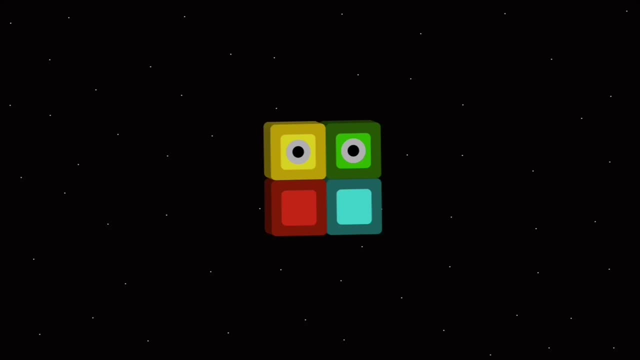 its three forces, electromagnetism and mass, would be the same If the super-symmetric particles were included in the standard model. the interactions of its three forces, electromagnetism and mass, would be the same. The super-symmetric and strong and weak nuclear forces can have exactly the same strength.